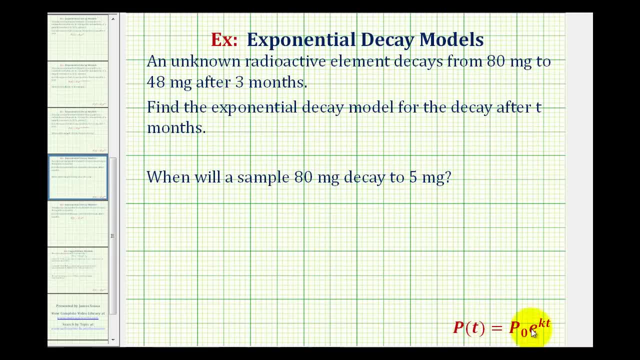 So to model this situation we'll be using the exponential growth and decay function. p of t equals p sub zero times e raised to the power of kt. where p sub zero is the initial amount or starting amount, k is the exponential decay rate. 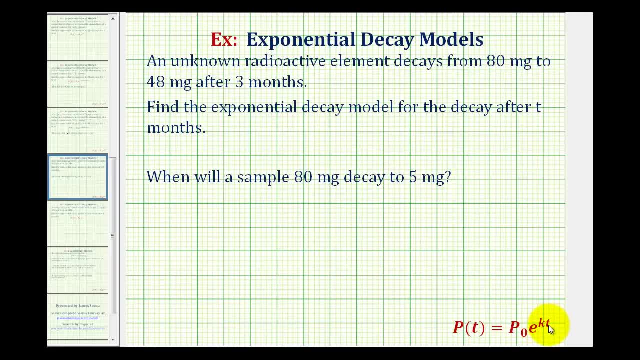 Since we have decay, k should be negative, T will be the time in months and p of t will be the amount of radioactive element after t days. So let's find the exponential decay model on the next slide. Reading this question again, we're starting with. 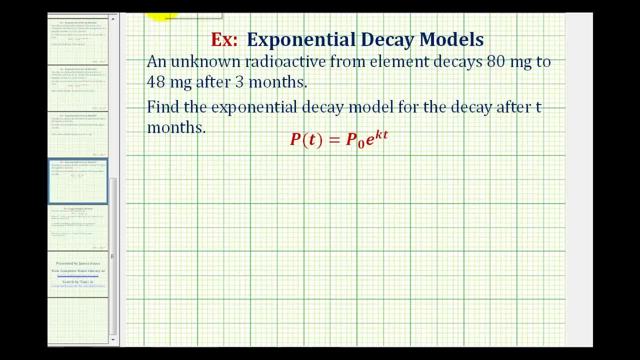 80 milligrams of radioactive material, which means p sub zero is equal to 80, or 80 milligrams. And then after three months we have 48 milligrams of radioactive material. So after three months, or when t is equal to three, 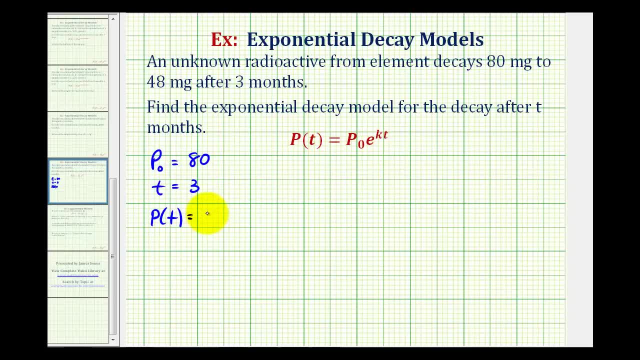 the amount of radioactive material, or p of t, is equal to 48. Now we can sub these values into our exponential decay function and solve for k the exponential decay rate. So we want to solve the equation. 48 equals 80 times e raised to the power of kt. 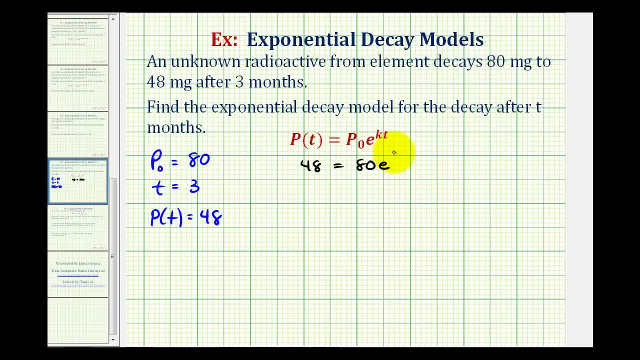 k times t, but t is three. so we have e raised to the power of 3k. And now to solve this, we want to isolate the exponential part, so we want to divide both sides by 80.. This simplifies to one, and 48 divided by 80. 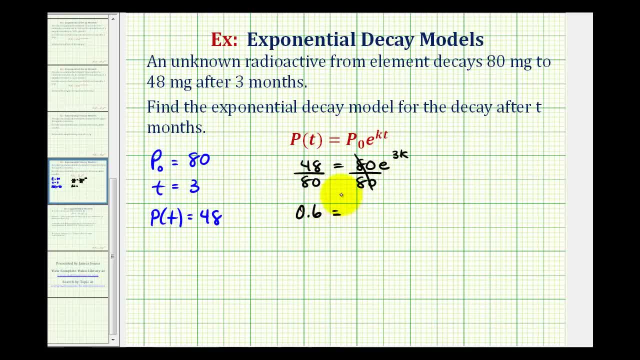 is equal to 0.6.. So we have 0.6 equals e raised to the power of 3k. And now we want to take the natural log of both sides of the equation so that we can apply this. We can apply the power property to the logarithm on the right. 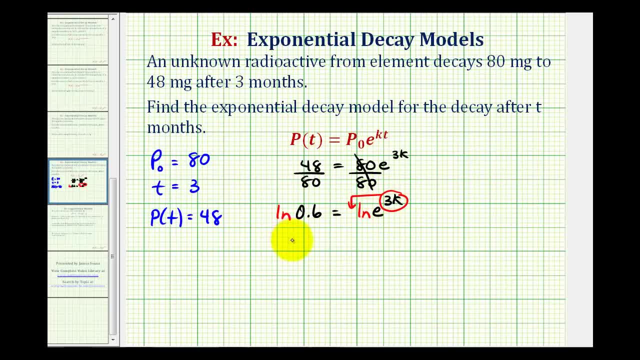 We can move this 3k to the front. So now we have the equation: natural log 0.6 equals 3k times natural log e, But natural log e is equal to one. Remember natural log is log base e And since e to the first power is equal to e. 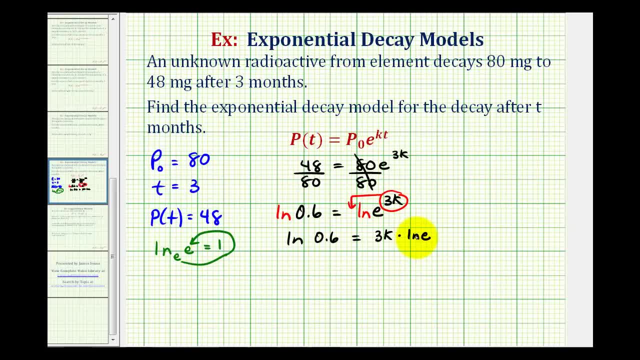 this is equal to one, And multiplying by one doesn't change anything. so a lot of times you'll see textbooks not even write this. So to solve for k, we just need to divide both sides by three, And now we'll get a decimal approximation. 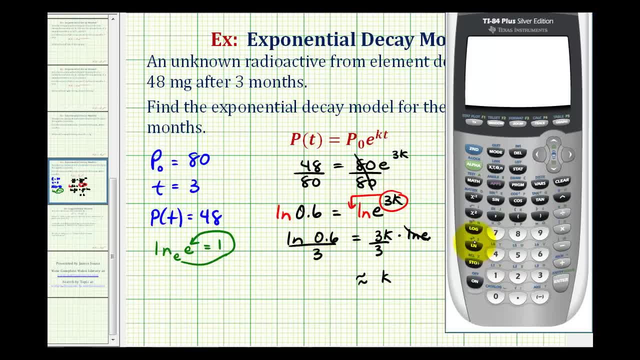 for our exponential decay rate. So we'll have natural log 0.6 divided by three. We do want to include quite a few decimal places for accuracy, so let's include six decimal places. So we're going to have k value of negative 0.170. 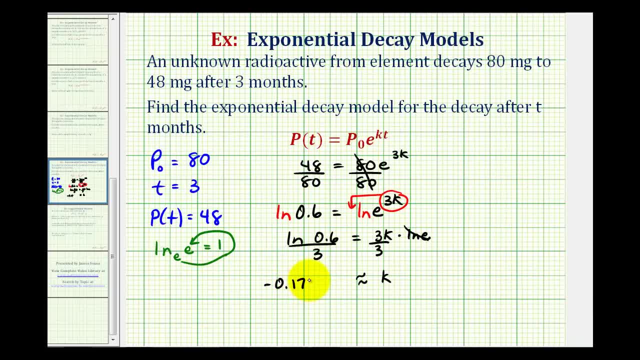 two, seven, five. And now we have the information we need to write our exponential function. We know that p of t is going to be equal to the initial amount of 80 milligrams times e, raised to the power of negative 0.170. two seven, five t, where t would be the time in months. 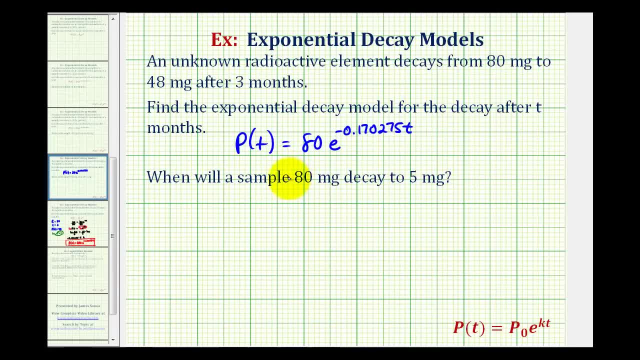 So with this function, if we knew the number of months that had passed, or t, we could determine how much of radioactive material would be left. But for the last question, we want to know when will a sample of 80 milligrams decay to five milligrams? 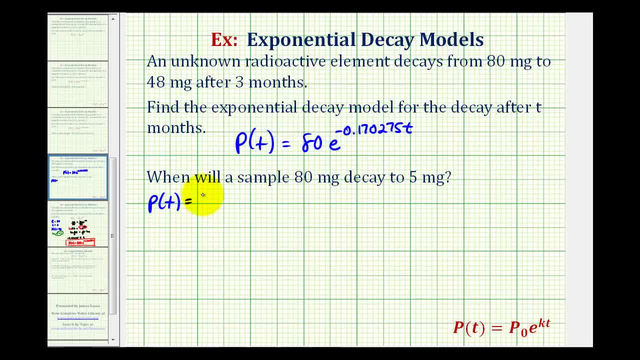 So they're telling us that we want p of t to equal five milligrams. We want to know t or how long this would take. So now we want to solve the equation. five equals 80. Times e to the power of negative 0.170. two seven five t. 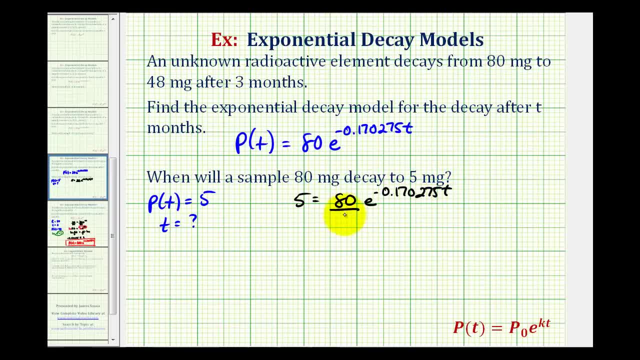 Now, this is very similar to the last equation that we solved, So we'll start by dividing both sides by 80.. Five divided by 80 is equal to 0.0625.. Just as before, now we'll take the natural log of both sides of the equation. 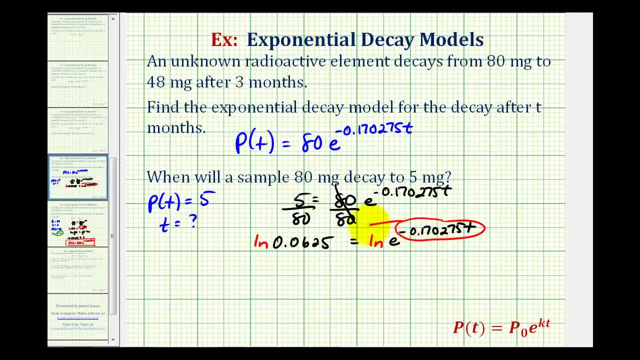 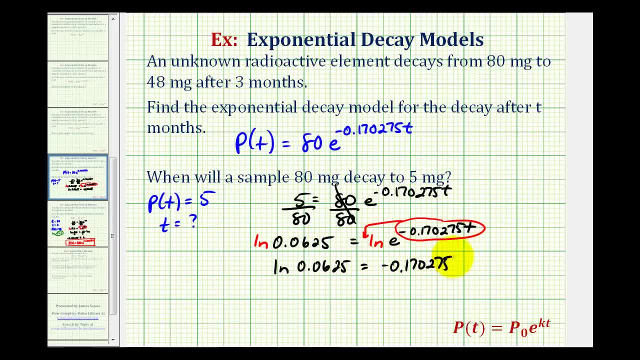 So we'll have negative 0.170, two, seven, five, t again times natural log e. but natural log e is equal to one. so we'll leave that off. And now to solve for t. we'll divide by this coefficient. This simplifies to t.